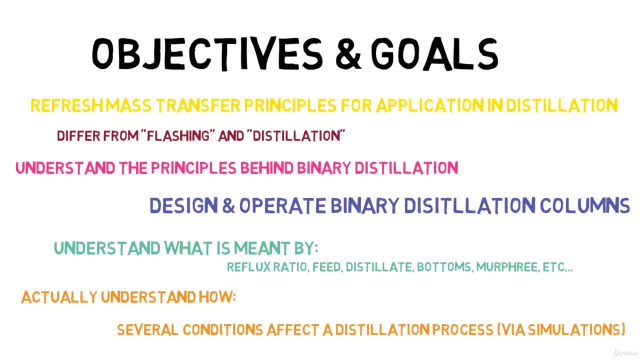 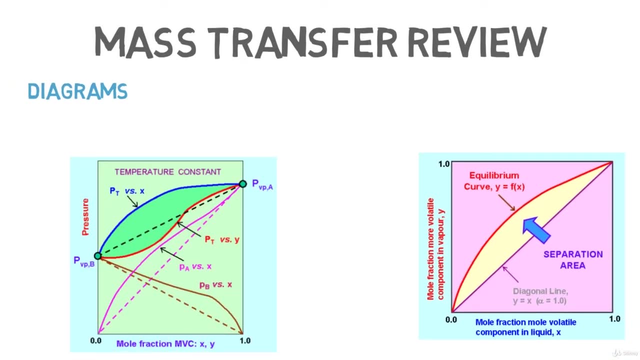 efficiencies, distillate-to-bottom ratio compositions and so on. All this is done via analysis of solved problems, exercises and simulations. First things first. we're going to start with a mass transfer review and we're going to start with diagrams. The most important diagrams in binary distillations are: 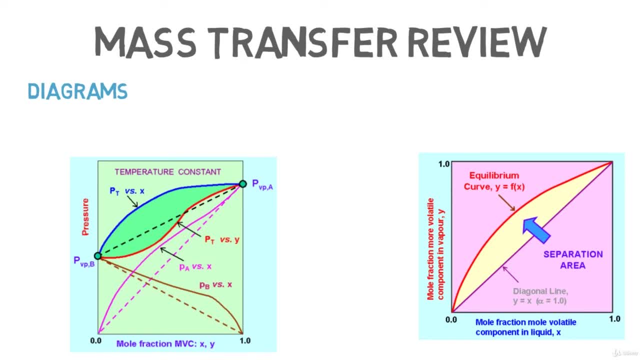 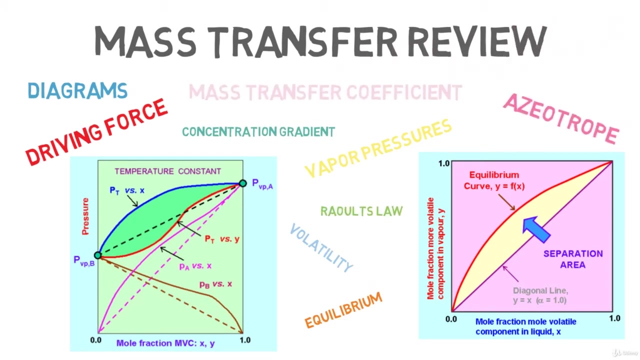 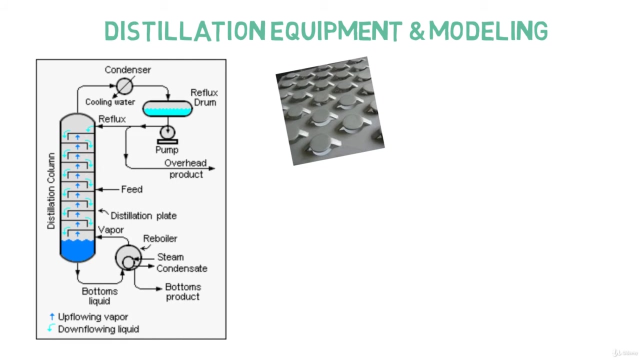 pressure versus composition, temperature versus composition and vapor versus liquid compositions. We then continue with vapor pressure, volatility, equilibrium. what is driving force? concentration gradients, Raoult's law, energy drops and so on. The following section covers distillation equipment such as sieve trays, valve trays. 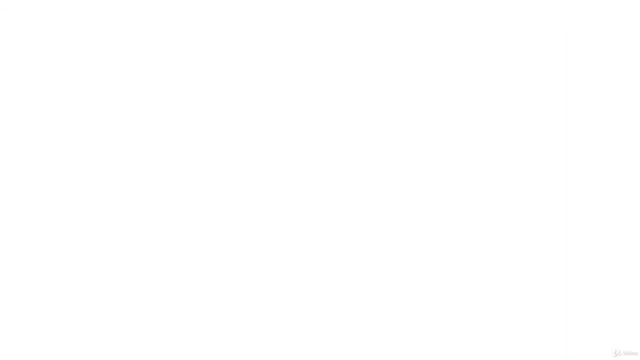 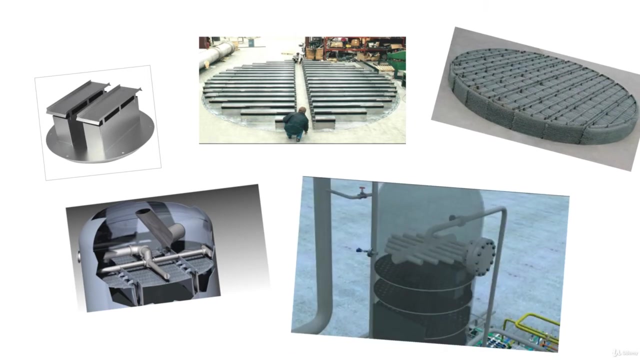 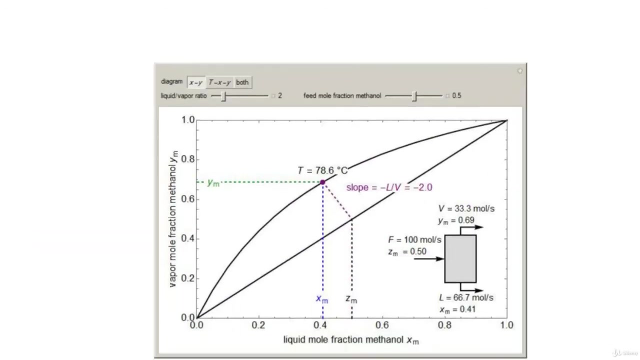 bubble cap trays. and not only that. we continue with deeper understanding of the column internals, such as liquid holders, redistributors, demisters and so on. Afterwards we continue with flash distillation. We get to know how to make energy and material balances using the TXY and enthalpy diagrams. 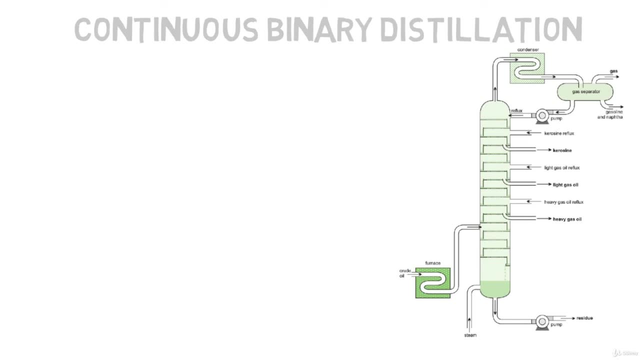 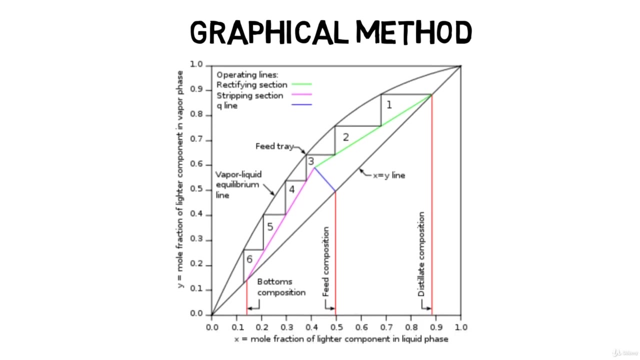 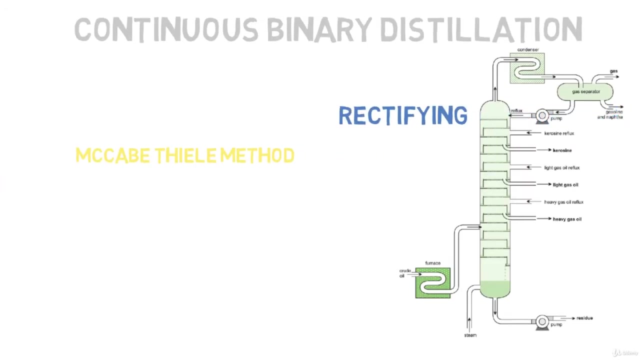 And now we're ready to model continuous distillation columns. We start with the McCabe-Diel method, which is a graphical method used to identify the total number of equilibrium stages that are required for a given process. We continue our analyses on the rectifying section, in which we are going to enrich or purify our distillate. 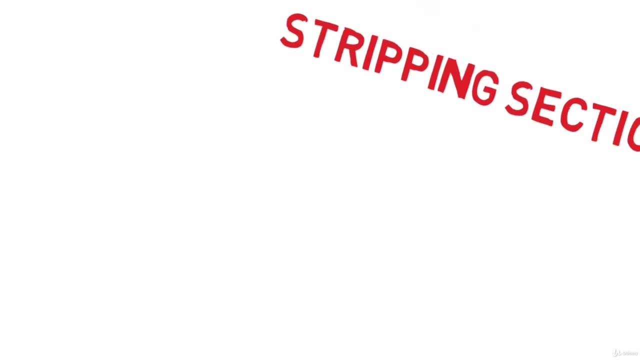 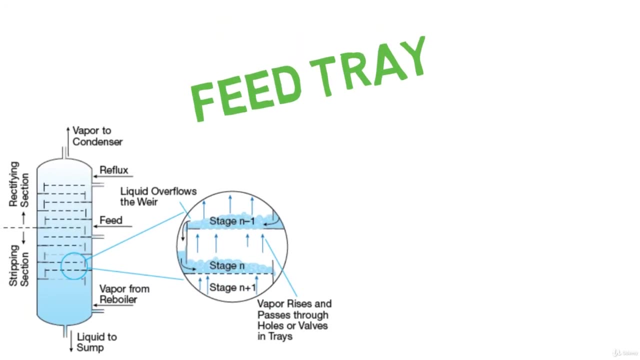 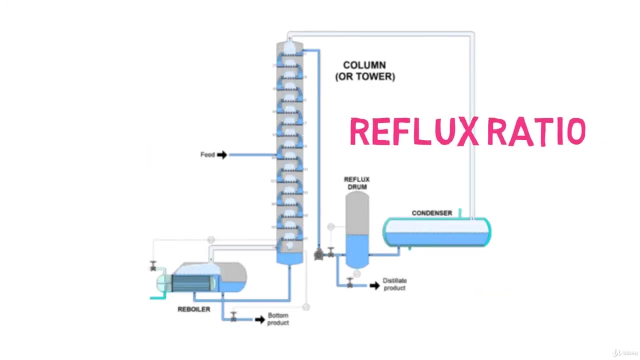 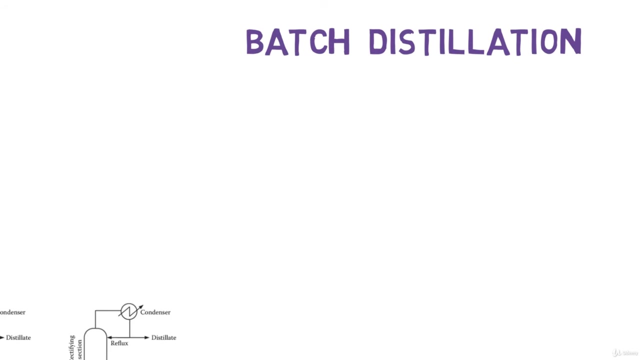 the stripping section comes next, in which we purify our bottom product and then we get to know what is the recommended feed rate for the complete feed of the column. then we verify the recommended reflux for our operation and eventually verify our tray efficiency. one of our last sections will be batch distillation, which is pretty similar to 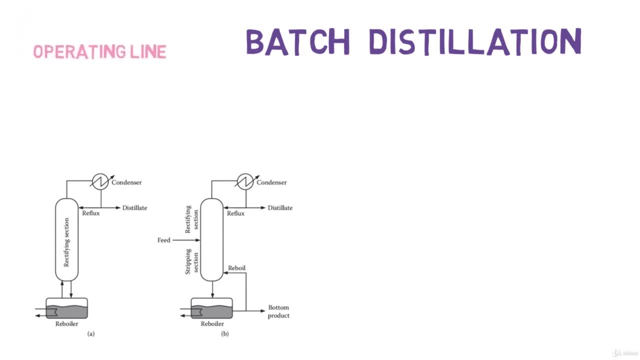 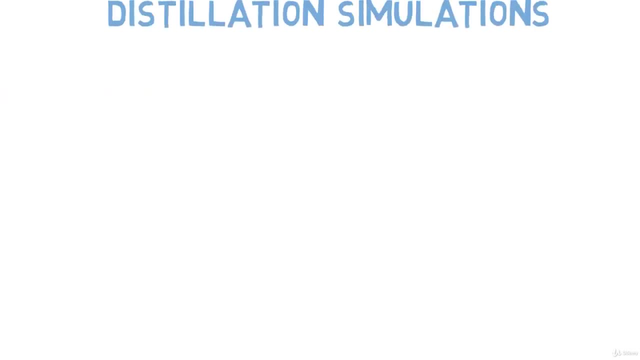 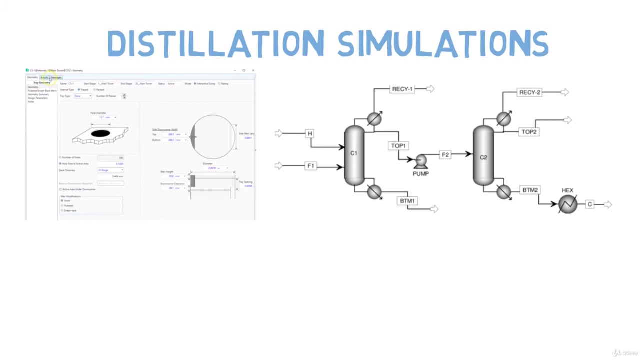 continuous distillation, in that we're going to be using a operating line, we're going to analyze constant composition versus constant reflux and, finally, we simulate several case scenarios. for instance, what happens when we change the type of tray or sizing, what happens when we change the recycle rate, the bottom rate, composition in the inlet feed tray, and so on. what happens when